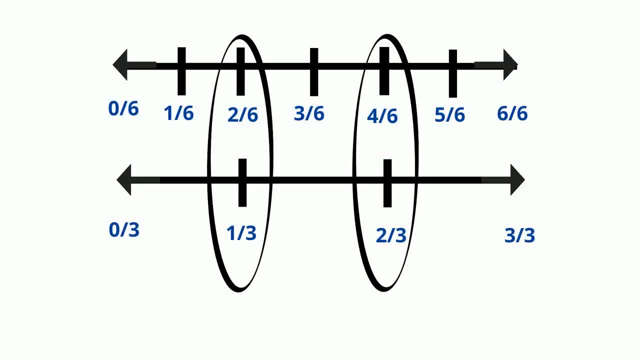 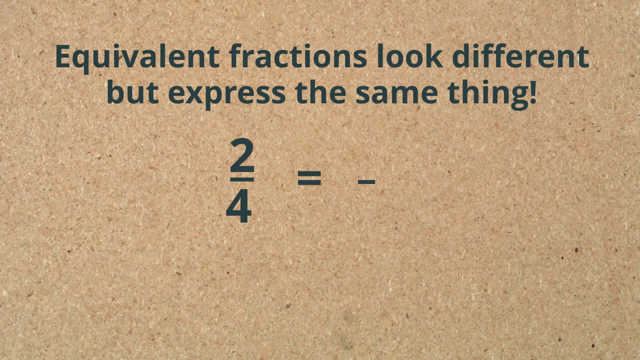 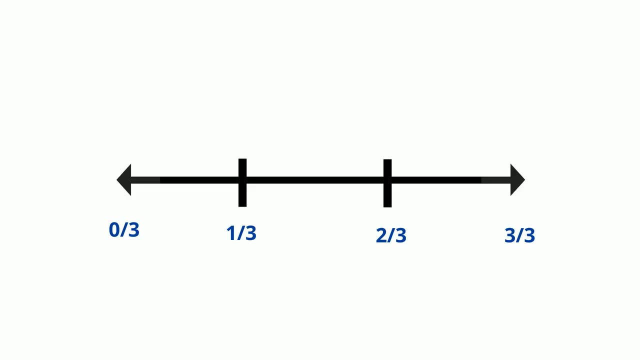 Welcome to MooMooMath and Science and equivalent fractions on a number line. Remember, equivalent fractions look different but express the same thing: 2 fourths and 1 half are equivalent fractions. Now to help you understand equivalent fractions a little bit more, let's take a look at some number lines. This first number line I have 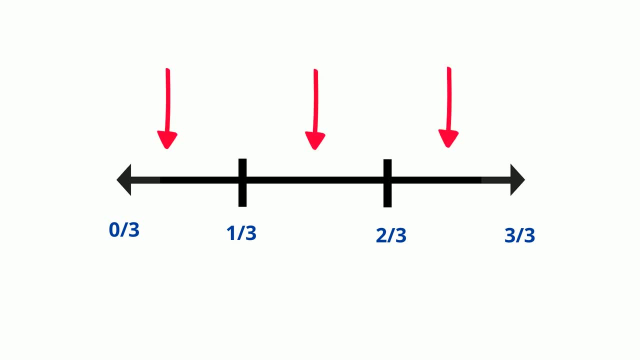 divided into three parts. We have 1 third, 2 thirds, etc. Now I'm going to take a number line of the same length and divide it into six parts. So now we have 1 sixth, 2 sixths, 3 sixths, 4 sixths. Take a look at 1 third and 2 sixths. They measure the same point. on the number, 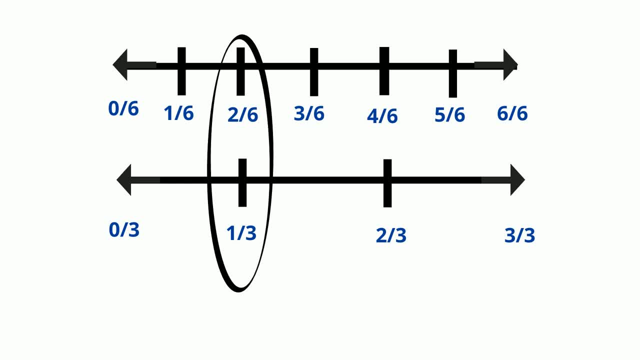 line. They are equivalent fractions. They measure the same thing, but look different. 2 thirds and 4 sixths measure the same point, So they also are equivalent fractions. Let's take a look at another example On this number line. I have it divided into 4 parts. 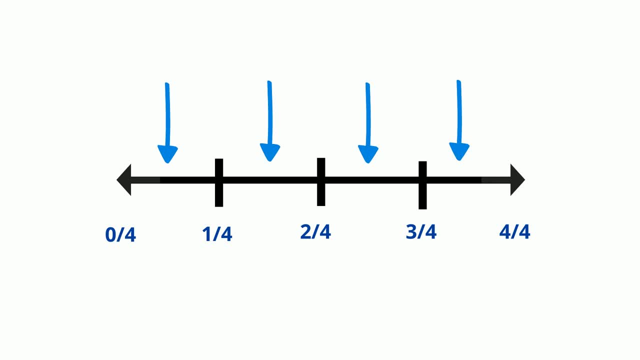 1 fourths, 2 fourths, 3 fourths. I next will take a number line of the same length and divide it into 8 parts. Again, take a look at 1, fourth and 2 eighths. They measure the same point on the. 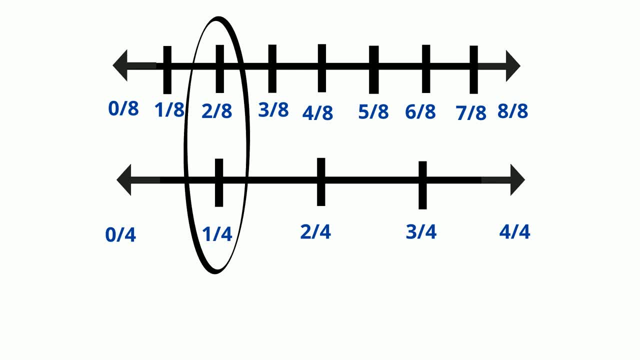 number line. They are equivalent fractions. 2, fourths and 4 eighths measure the same point. Equivalent fraction. Look different but measure the same thing And the same with 3, fourths and 6 eighths. Now I'm going to divide the number line into 16 parts And it's small. In fact it's so small I. 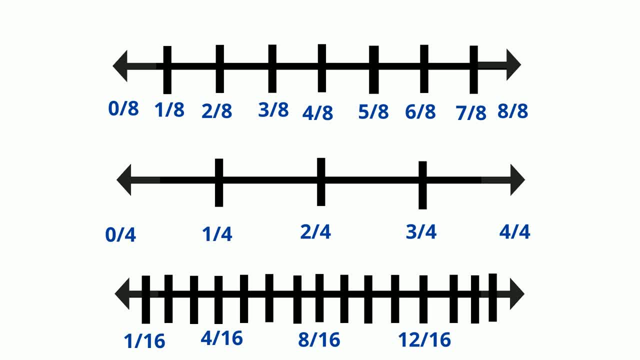 couldn't put the fractions on the bottom. It got too messy, So let's count them off. We have 1 sixteenth, 2 sixteenths, 3 sixteenths, 4 sixteenths, 5 sixteenths, 6 sixteenths, 7 sixteenths, 8 sixteenths. 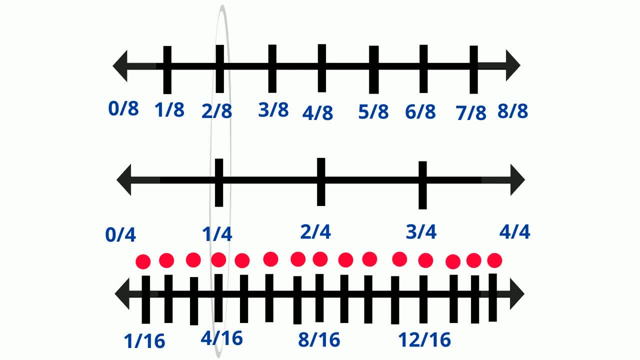 etc. Now again, let's take a look at 1- fourth, 2 eighths and 4- sixteenths. They all measure the same point on the number line. All three of them are equivalent fractions. Now let's move over to.